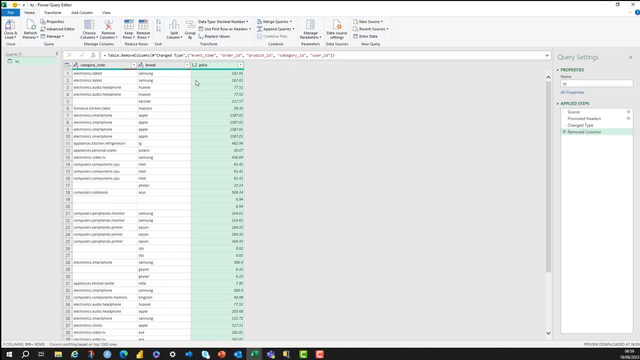 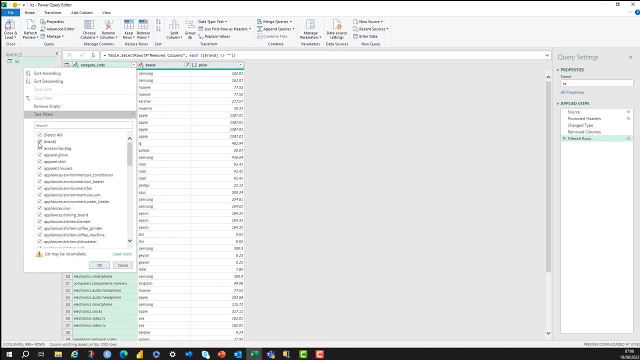 and then i'm going to go to remove columns and that leaves me with only the columns i want. next step is: i just want to get rid of blanks out of here, and no point in having blanks in this example, so i'm just going to filter the blanks out and press ok and then this category code i want: 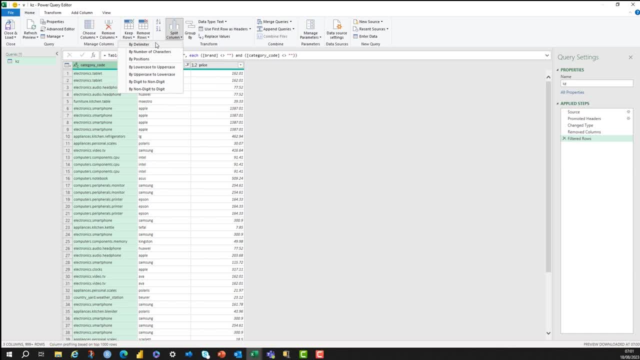 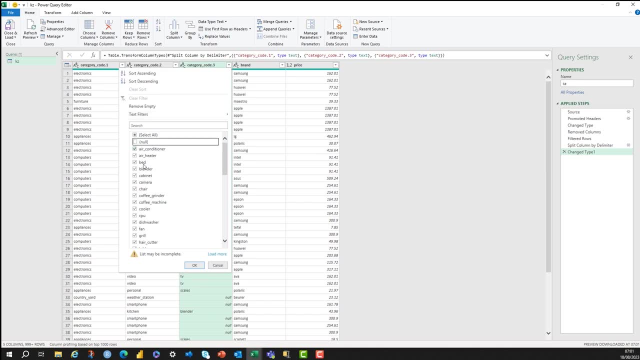 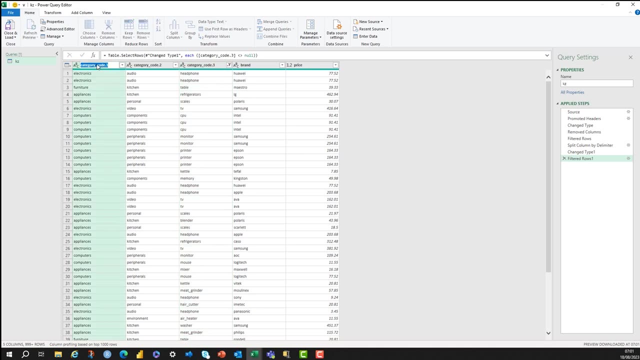 to split this into its different categories. so i'm going to do this by a delimiter at a full stop and then this is splitting this out into the three different parts of the category code. again, i'm going to go in and get rid of the nulls because i'm doing numerics in this video. i'm doing this very fast, but i'm just going to. 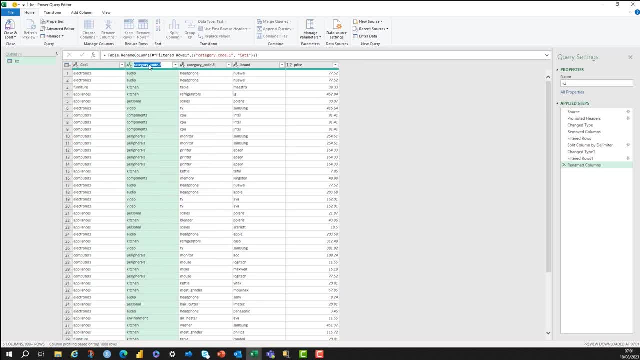 rename the columns here and then we can just start working on some of the numeric functions. but i will be doing a text video where i'm going to be going through all the splits and all that stuff in a lot more detail. so i'm just changing these three columns to cat1, cat2, cat3. i just want to talk. 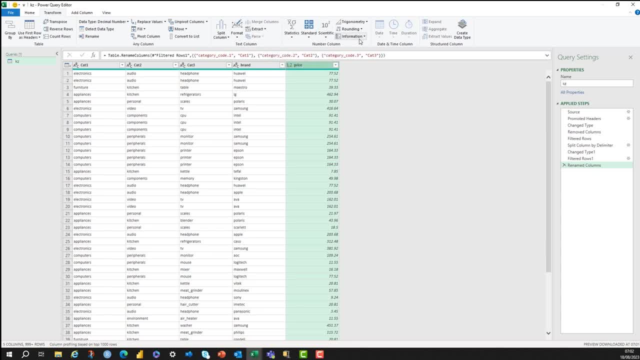 about the difference between the transform and the add column section in power query. so i'm going to go into the transform and the add column section in power query. so i'm going to go into the transform and the add column section in power query. so that's transformed there and this is add column and they both have. 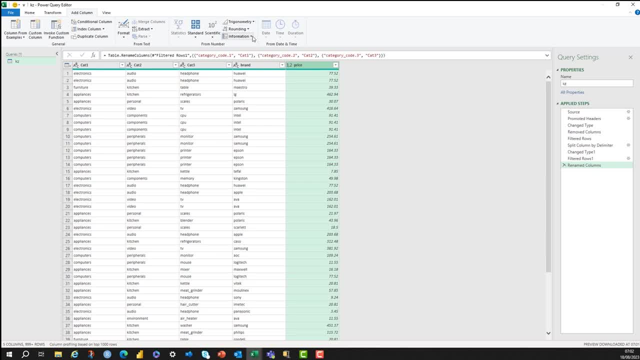 the numeric from numbers transformations. so in the add column information, i can just do a transformation to see what sign something has. it will come up zero and one. and then there's another inbuilt transformation and information which is odd, or even so is odd, and that'll come. 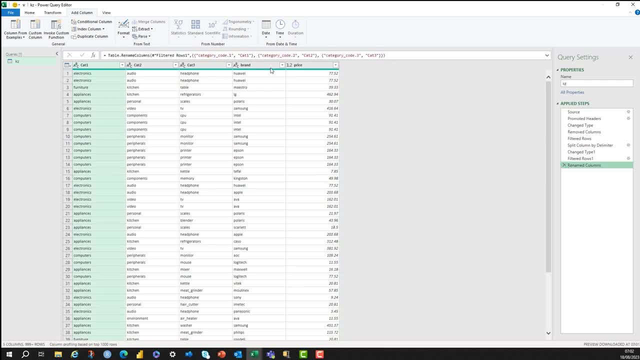 up with a boolean column there. next thing i'm going to do is i want to do some arithmetic, so just want to show you the difference between the transform and the add column here. so if i go to transform and add, this is going to add to the number in place, so i'm just going to add two. 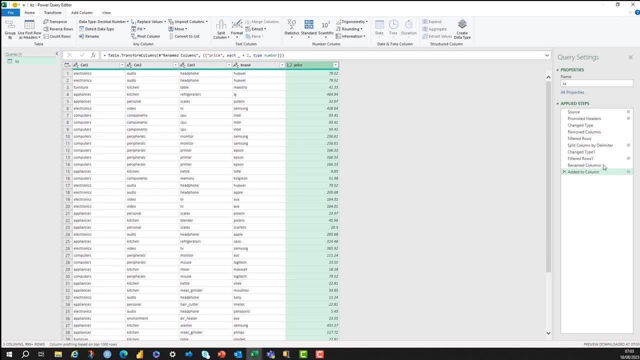 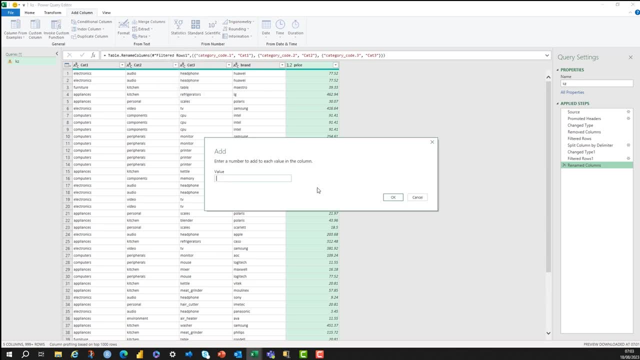 here and this has changed my price plus two. i'm going to just remove this here. if i do the same thing in add column, this will create a new column with two added to my number, so this creates a new column here. i'm going to multiply the price by 0.9 and this is going to stand in for my cost as you. 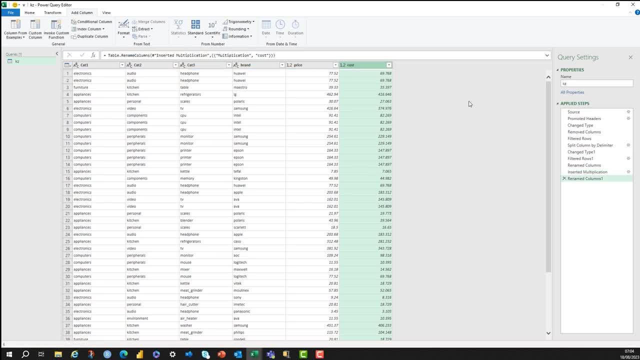 can see, there's three digits here, so i'm going to add two here and this is going to stand in for my cost digits here. so what i can do now is use the rounding functionality in the transform. so that's going to round it in place, and i'm just going to round this to two decimal places there's. 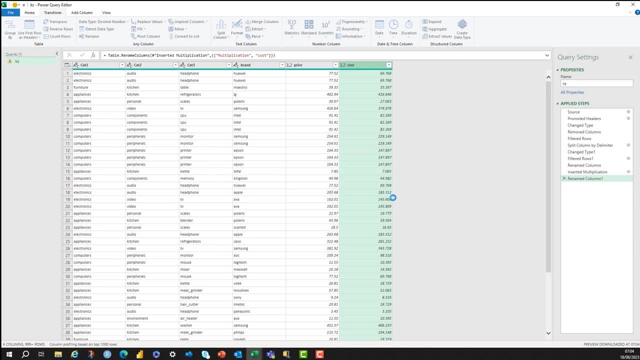 round up and round down options, but the round is probably the best one. i'm going to round that to two decimal places and then what i want to do is: i want to select my price, select my cost, go to add columns and select, subtract. so it matters what order you select them in. i select, selected, my. 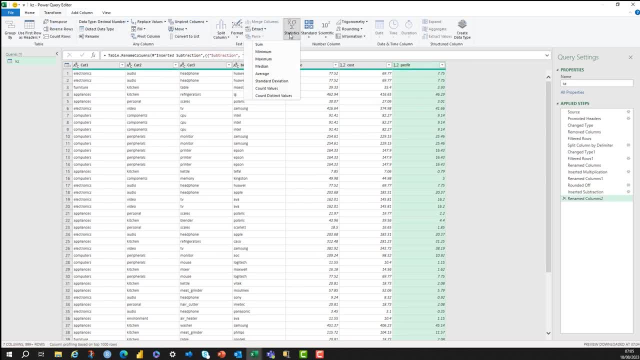 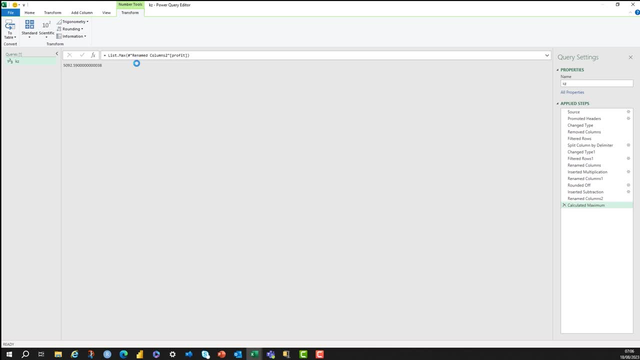 price, my cost, and then i was able to subtract in the aggregations. this is quite weird, right? so you've got all these aggregations in here. i'm just going to pick maximum in here, and this just creates a maximum number, and now that's the whole query, so that 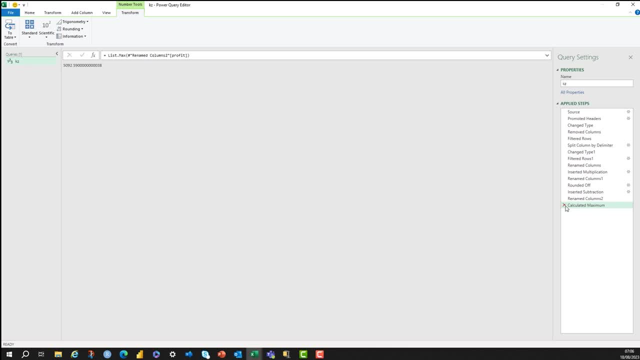 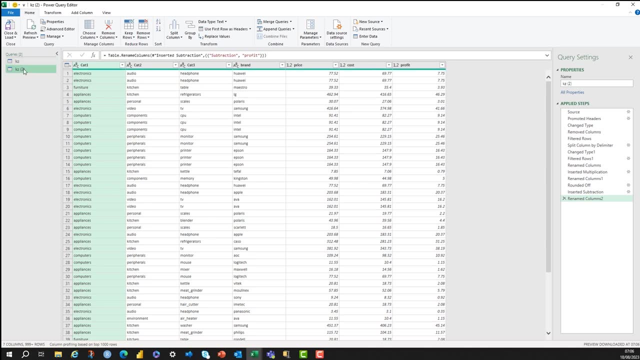 doesn't really work for me, but there is a trick you can do here. so i'm just going to get rid of that and i'm going to duplicate this whole query here and i can change the second one into just the maximum here. so i'm going to rename the second query max, and this is another query stands on. 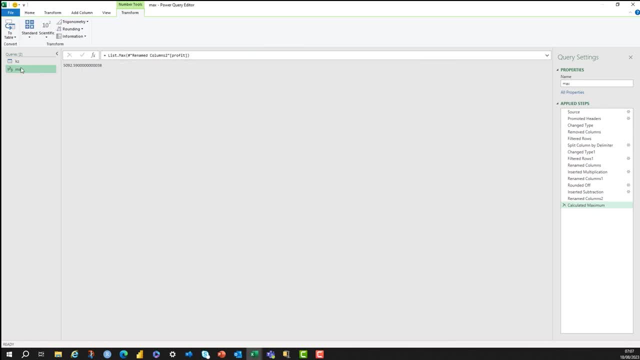 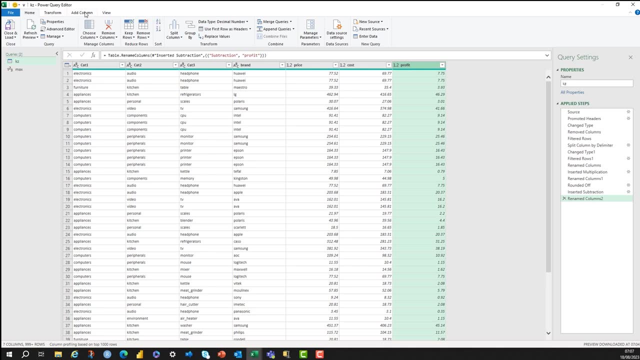 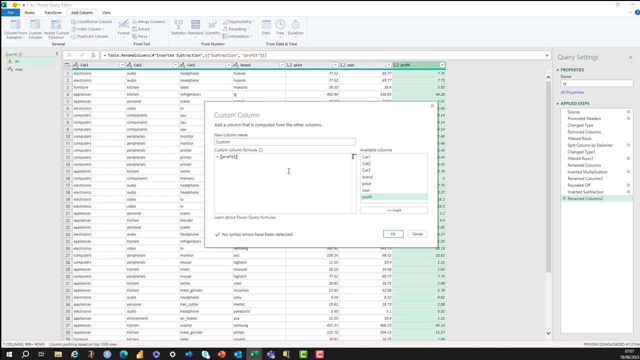 its own. i'm going to change this to maximum and now this is my maximum number. what i can do in the original query is i can reference that maximum calculation so i can go into add column, custom columns and i can create a conditional column here. i can call a profit and then minus max, and that's referencing the other query there. 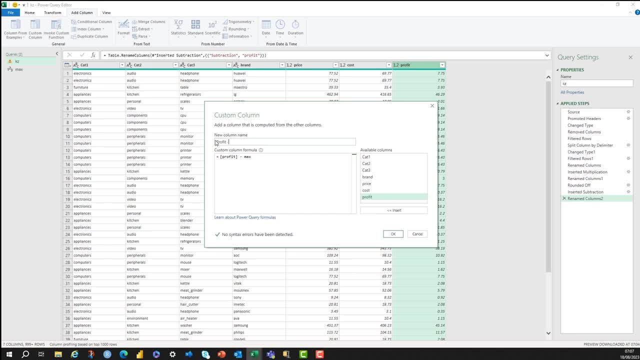 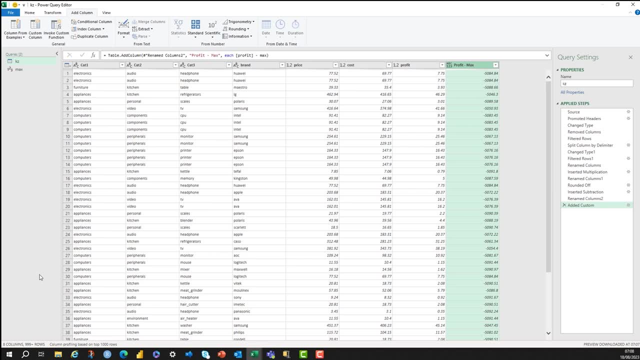 so minus the maximum, and then i'm going to rename that profit minus max, i'm going to select, ok, and that's actually brought in the aggregation as a calculation into my data set. so quite useful there, but what we would actually do in this instance if we wanted. 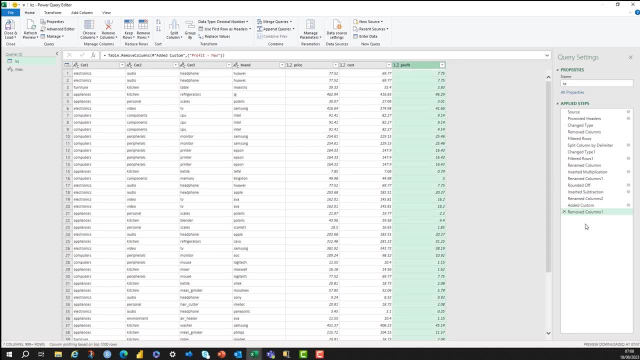 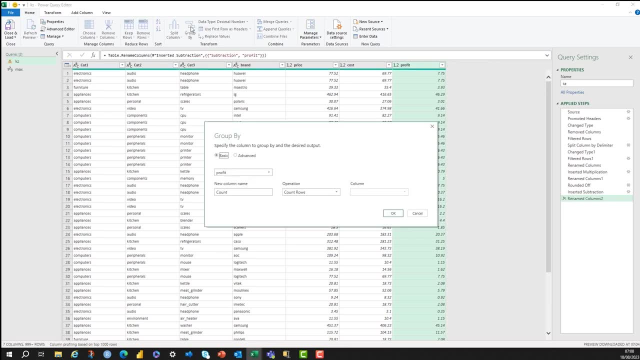 to group by data- we wanted to have aggregations- is we would use the group by functionality. I'm just going to clean out these last few steps here and I'm going to go to group by, and what I can do in advanced group bys is I can select a couple of columns to group by. so I'm going to add three. 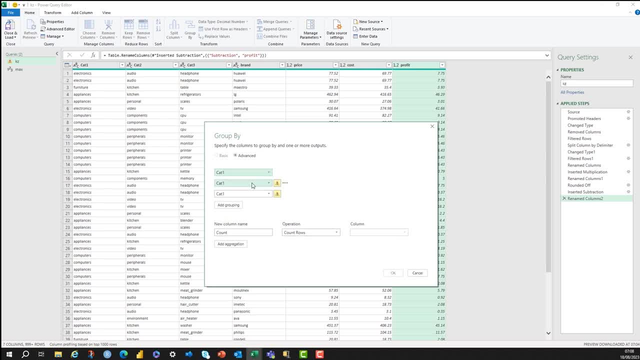 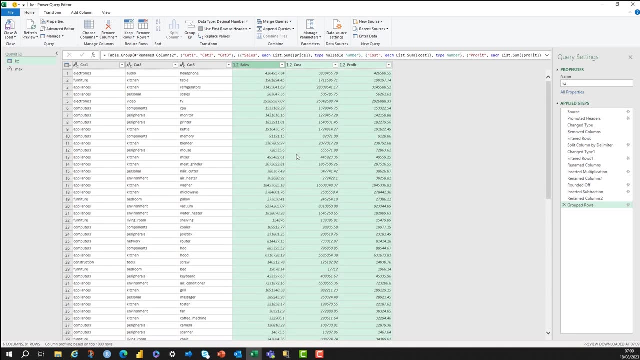 groupings. I'm going to add cat1, cat2 and cat3. this is going to form the basis for my output at the end of this. so cat1, cat2, cat3- I'm adding three aggregations here, just a sum of sales, cost and profit, and this will transform my query the way I want it now. so this transforms my query into just 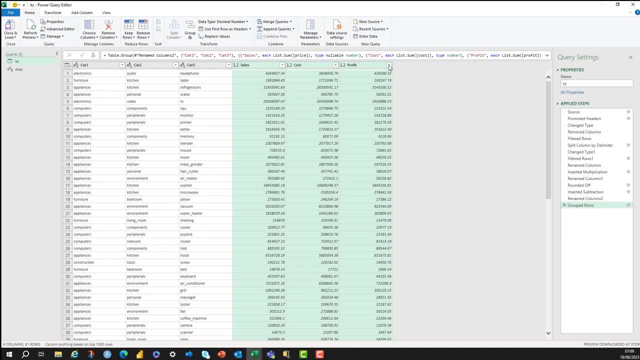 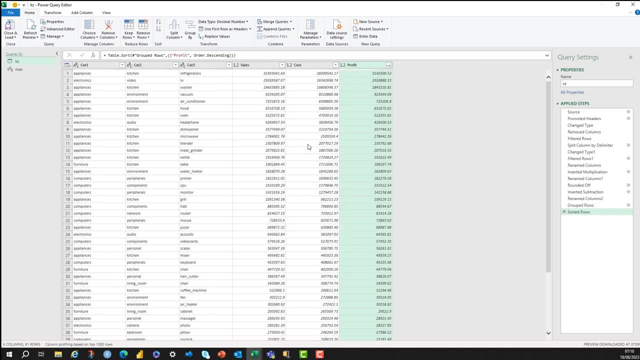 the three categories, the sales, cost and profit, and I can sort by just going into the column and sorting descending here. so this is sorted descending. I want to add another grouping in here because I think it'd be a good idea to have the number of transactions so I can just again. 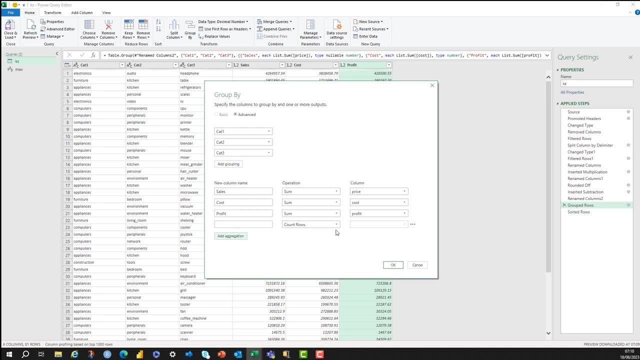 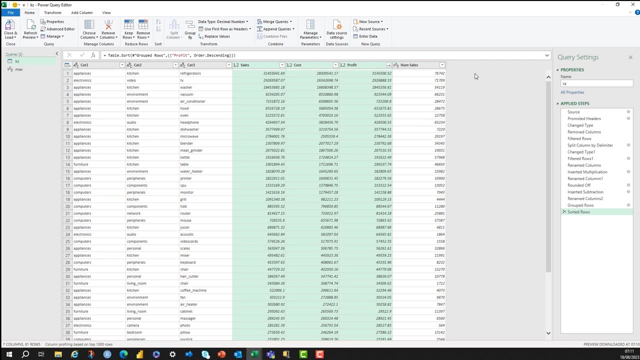 press the dial and I can add another aggregation, and this aggregation is just going to be count rows. so I just need to name this and I can just call this number of sales. I can press ok in here and this will give me a number of sales for each aggregation. so I'm good to go now back into excel. 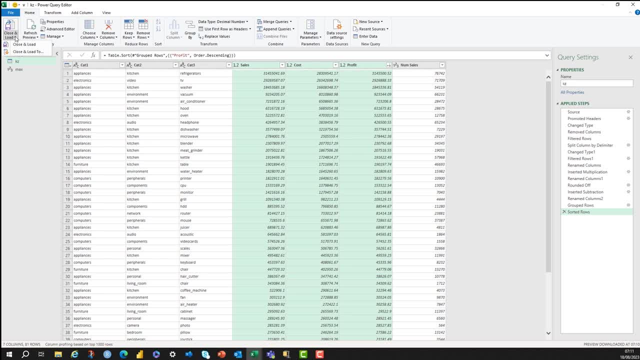 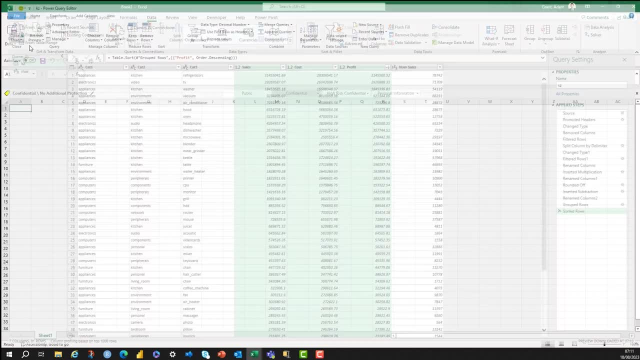 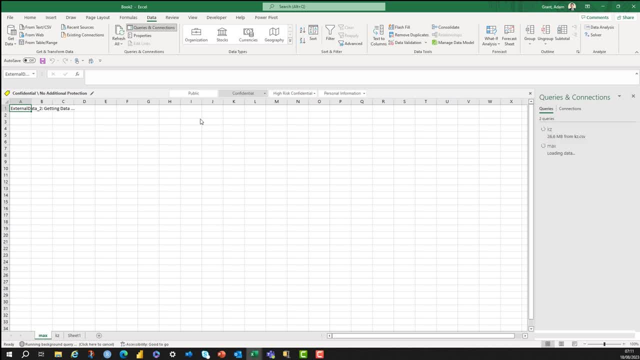 my max in there. if I need to do that to do some something else in my excel spreadsheet, I have my main query in there as well. so you see, these take a long time to load. so I've just sped up the video a bit. max is loaded and now the main query has loaded in here. so I've taken that very large. 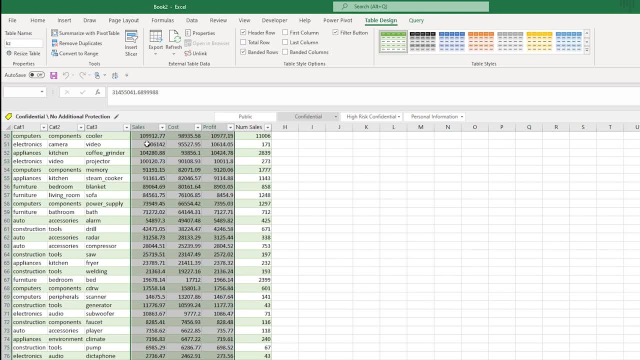 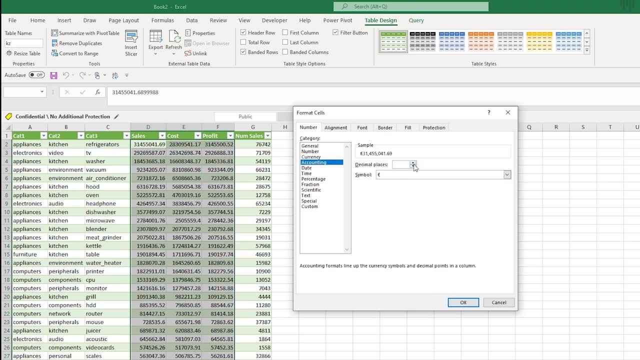 data set down to 81 rows. I've got my aggregations. I can just do my formatting in here. next time we're going to be looking at text transformations, which are probably the most used transformations, but in power query I'll put a link up to that one in the description below. so if you're interested in,